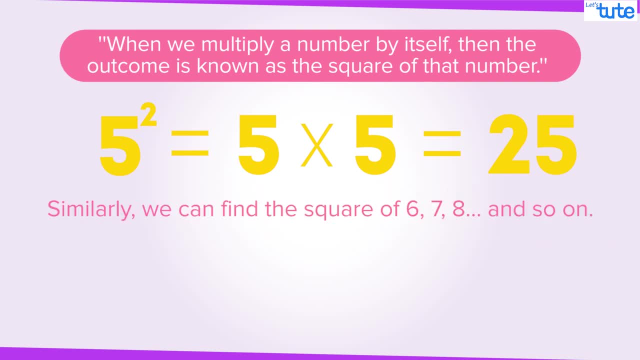 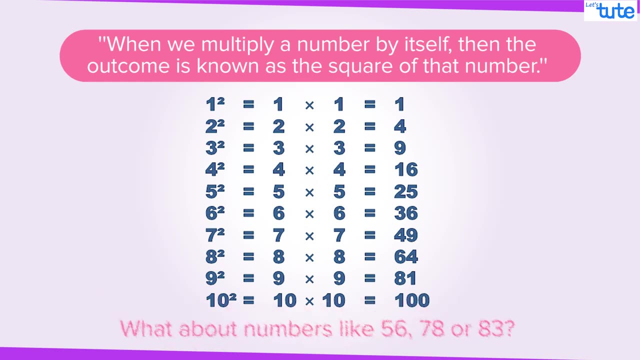 5, which is equal to 25.. Similarly, we can find the square of any number. Most of you must be knowing squares of numbers from 1 to 10.. But what about numbers like 56, 78 or 83?? It is tedious, difficult and time consuming to find the square of any big number. 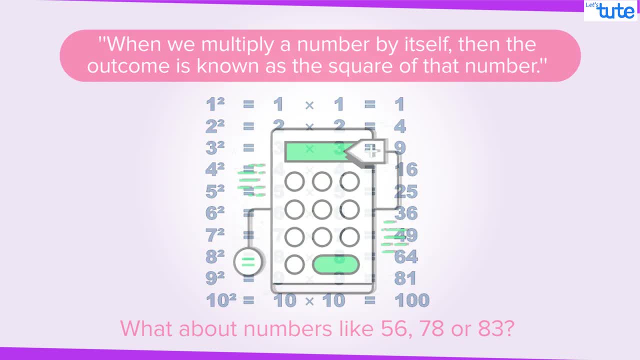 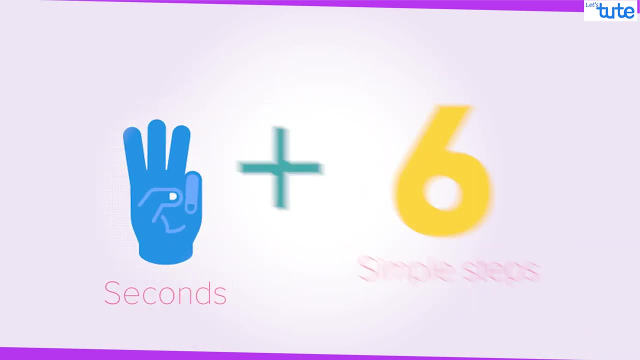 especially when you don't have a calculator lying around, right? So here we are with the solution and some tricks to find the squares of any number in just 3 seconds and 6 simple steps. Yes, friends, you heard it right. So, without wasting any time, let's start our. 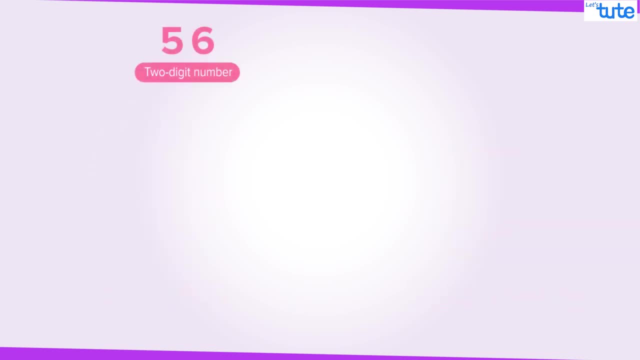 session Now. 56 is a 2-digit number. The square of this number will be in 4 digits Here. first number is 5.. Square of 5 is 25.. Next number is 6.. Square of 6 is 36.. 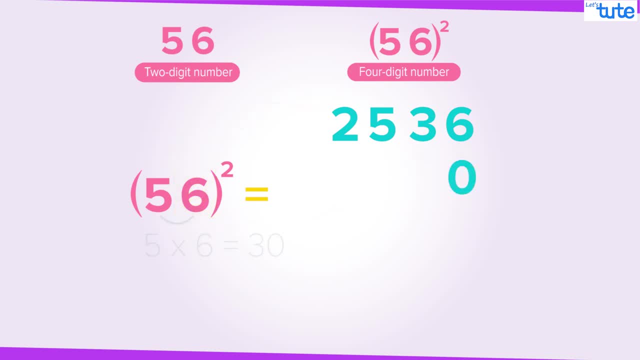 Now write down 0 here. Now 5 into 6 is 30.. Multiplying 30 by 2, which will give us 60.. Write 60 here. By adding these two numbers, ie 2536 and 600, we will get 3136.. Therefore. 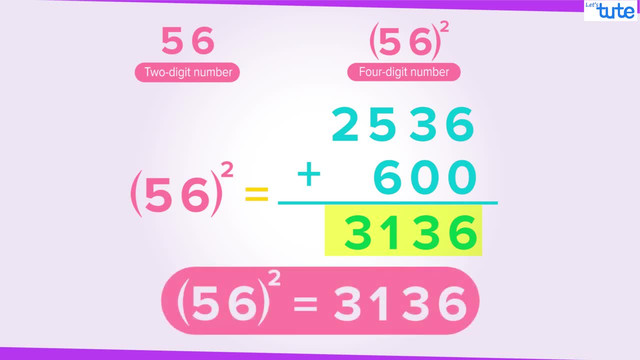 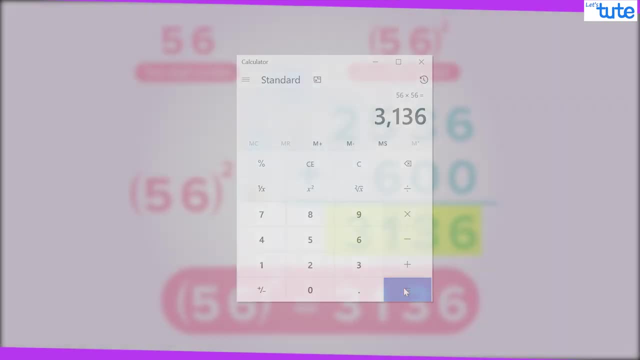 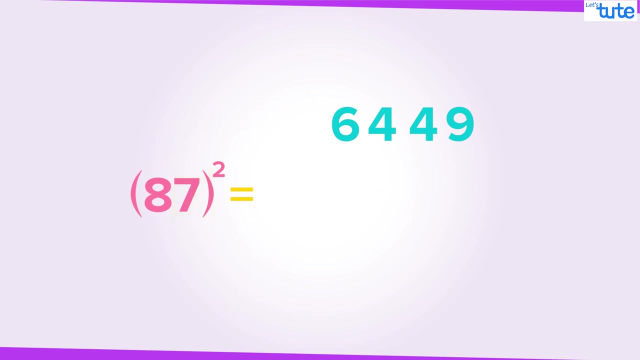 square of 56 is 3136.. We can check the same in the calculator too. Well, the answer will be the same. Let's try the same with another number, Let's say 87. And let's repeat the same procedure. Square of 8 is 64.. Next number is 7.. Square of 7 is 49.. Now write. 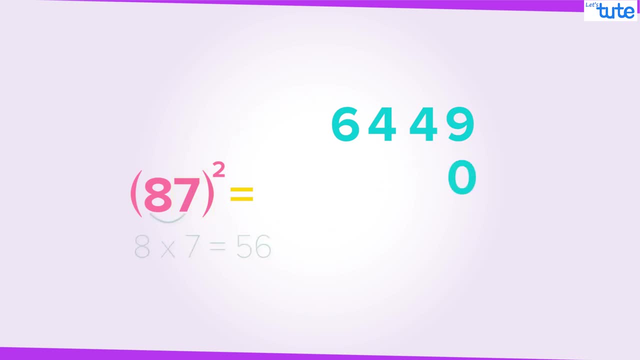 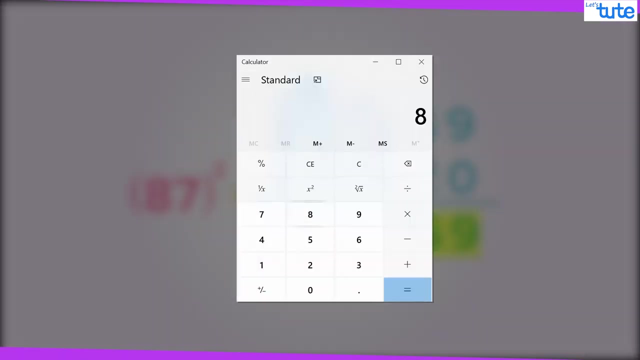 down 0 here. Now 8 into 7 is 56.. Multiply 56 by 2, which will give us 112.. Now write here: 112.. Now, by adding these two numbers, we will get 7569.. Let's see what the calculator. 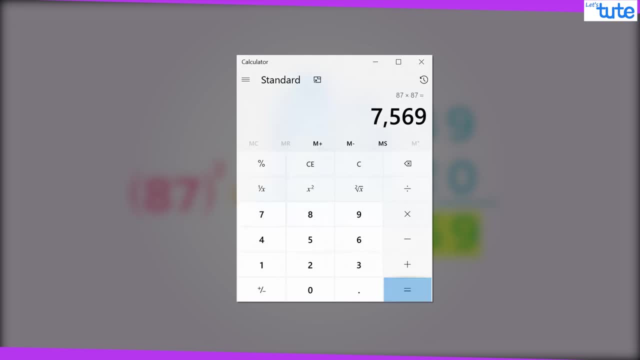 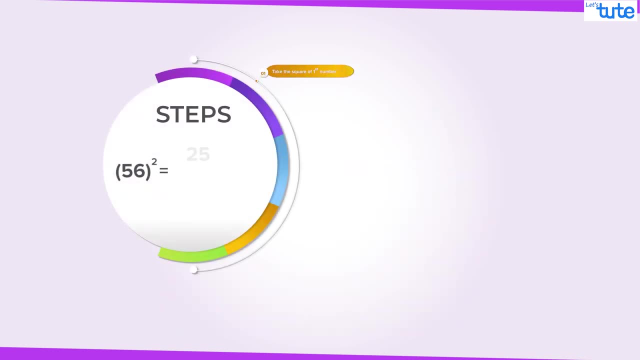 says: Well, the answer is correct, Isn't it amazing? Well, guys, let's just go through the steps once again. First step is: take the square of the first number. Second, take the square of the second number. Add a 0 below the last digit. Fourth, multiply.